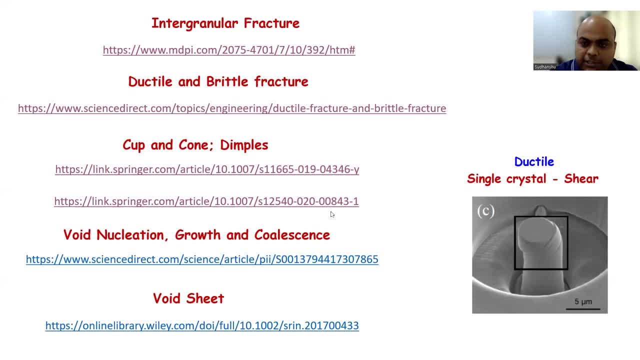 Okay, so let's begin. So the first one, what you see here on the right side is for ductile material. This is a single crystal and, if you remember, we were talking about this in the first lecture. if I am correct that if you are doing uniaxial tension and it is single crystal, then they will be shared. 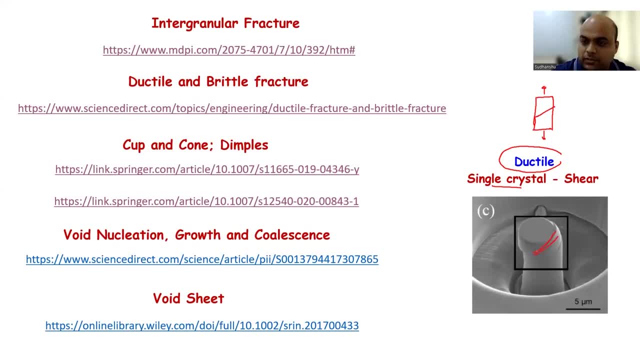 Right, and this is what you observe here. So you see, it's here along these planes. Okay, so these are actually pillar compression. Okay, these are very small in size and we can see that they are very small in size. So we will try to understand the effect of size, sample size also when we do pillar compression. 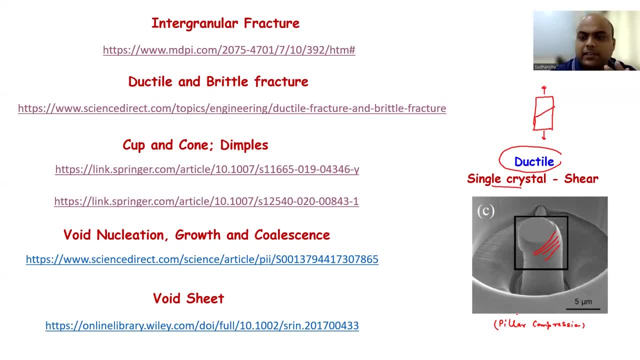 Nevertheless, if the sample size is also large, but if it is single crystal, it is going to show you the same behavior. Okay, now let's see how intergranular fracture is going to look like. So what I have done- I have different links here, and I'm these: 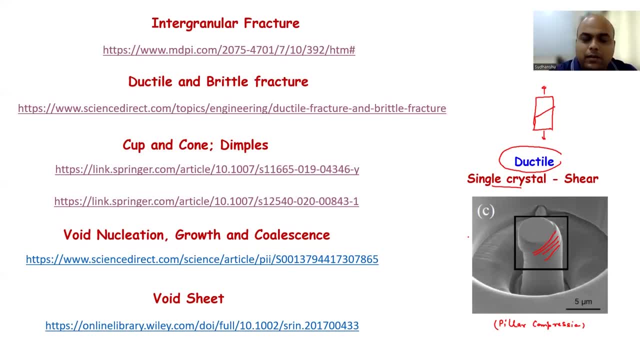 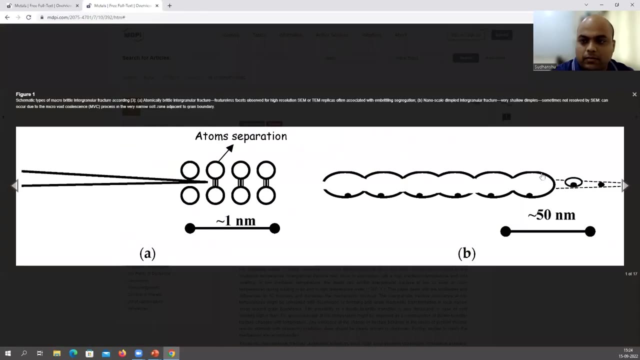 links will take us to the online paper where I will be showing you all the microstructures, or micrographs. Okay, So the first one is intergranular fracture. Okay, so if you see here, some more stuffs are here, right, So you can see. 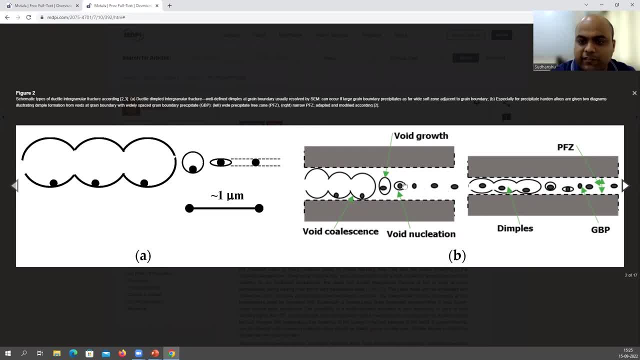 these are inclusions, Okay. then you see void nucleation is taking place in this particular inclusion, Then you have void growth and then finally void are getting molasses, Okay. so this system, systematic, shows very nicely the three parts: nucleation, growth and prolessions. 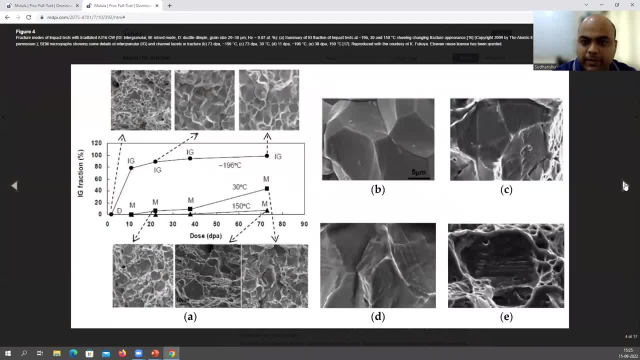 all together. Now let me bring to the intergranular fracture. Okay, so this particular image here at the center, this is intergranular fracture. What you see here is a typical brain. Okay, so whenever we talk about intergranular fracture, remember the track propagates through the 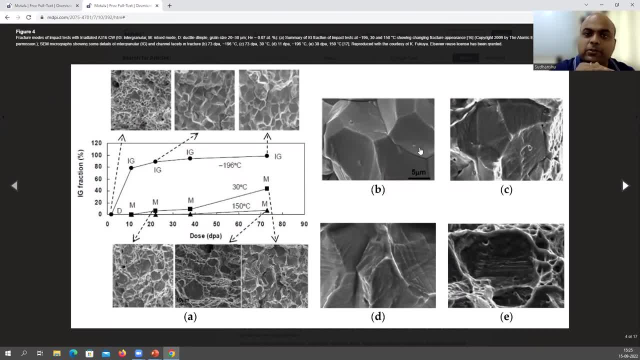 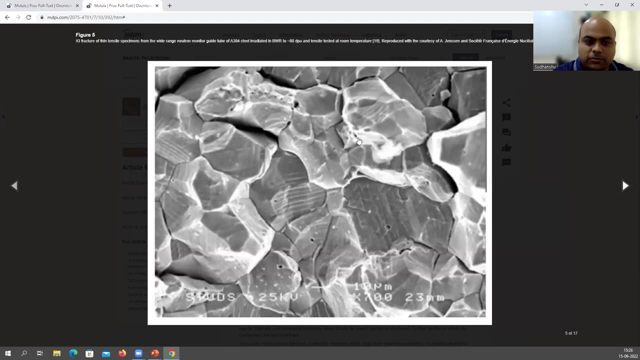 grain boundary. Okay, This fracture surface. if you are going to look like you're going to see the structure of drains, you're going to see the drain structure and that is what you see here here in this image and this image also. Okay, Yeah, So this is what I wanted to show. so what? 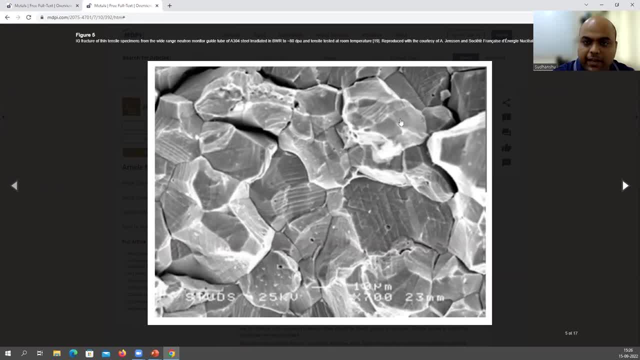 you see, here is this is like one drain, one drain, one drain. So the fracture surface, you know, is showing you the grain structure. Okay, this means that the track has propagated to the grain protection. It goes down of the field. So 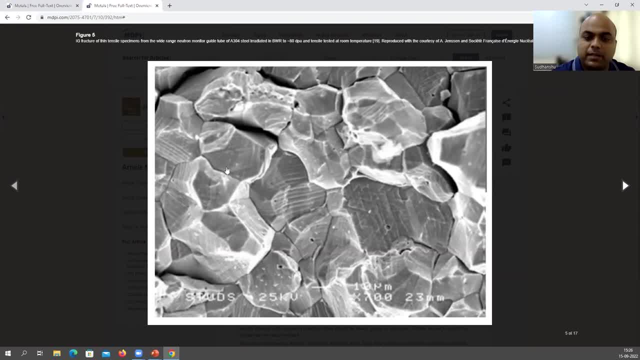 So So again, if you see this two side of it, it will be again any structure and it adds goes down of it. okay, because this will be another straw after that. Okay, So what are you see? such grain boundary? so this is typically how inter granular fracture surface is going to look like. 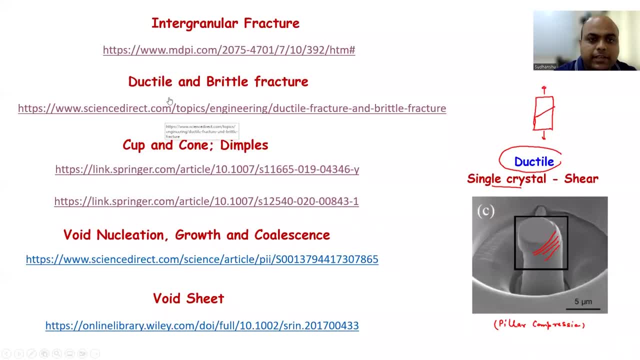 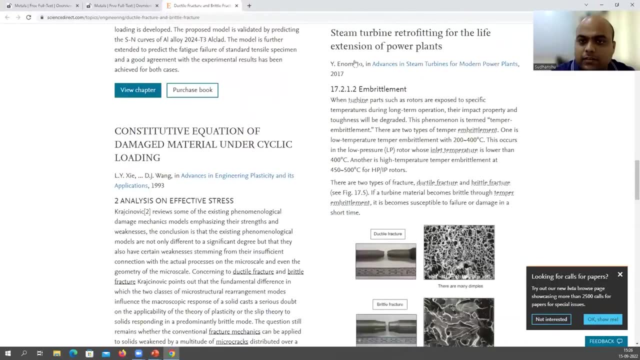 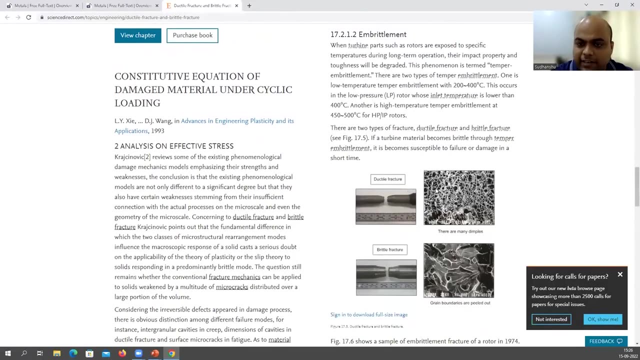 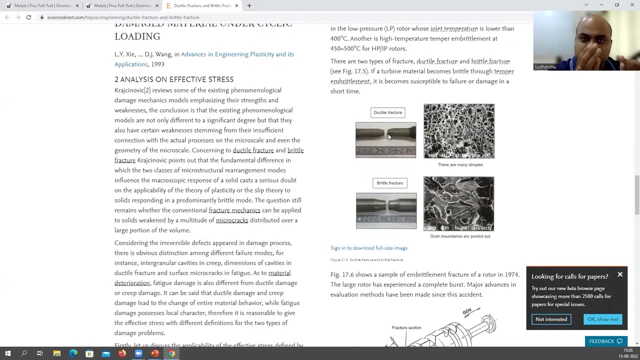 okay, now let's see ductile and brittle fracture. okay, so this is another chapter on steam turbine retrofitting for the live extension of our plant and it nicely shows both right ductile fracture and brittle fracture. you can see here and if you just see the ductile fracture, if you just open it, you will typically see cup and cone failure. 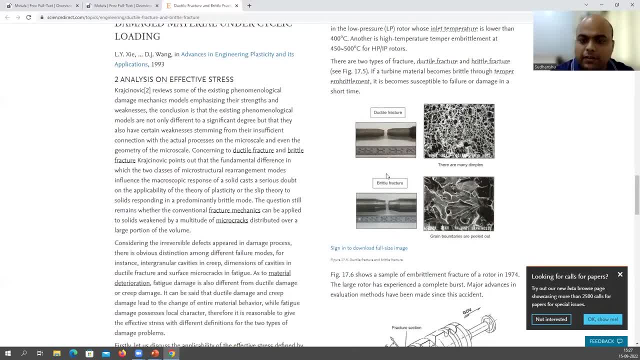 and the surface is going to be rough, whereas brittle failure- it will be like a brittle, it will be like a cleavage or a flat surface. okay, here also you can see dimples and these are your river patterns, but i'm going to come to that later. okay, so this is what i wanted to show in terms of 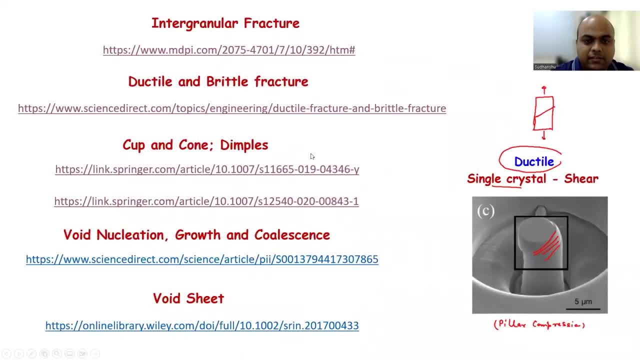 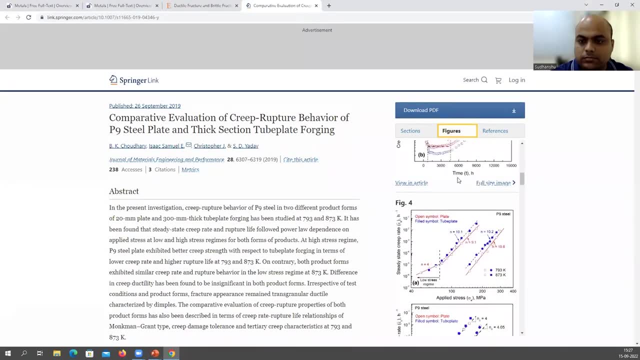 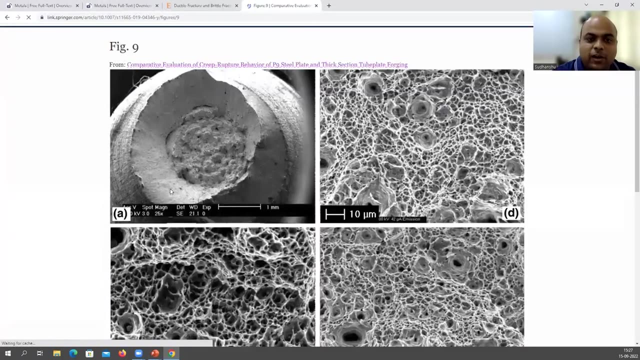 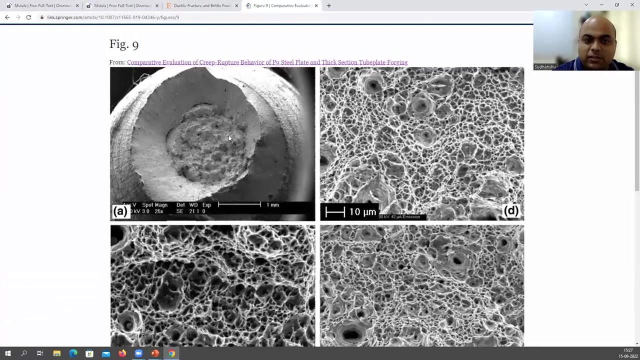 ductile fracture: ductile fracture and brittle fracture. now the next is cup and cone and dimples. okay, so this is how you know a cup is going to look like. okay, so you can see here, this is your fibrous zone at the center, which is a flat region, rough, and then you see. 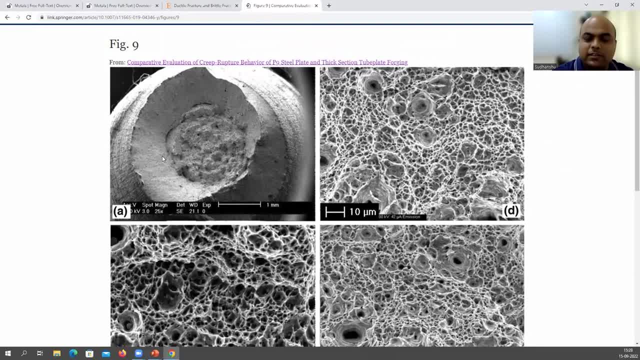 here, slant one, the shear lip, okay. so this is typically his cup and cone fracture, and what i have shown here is a cup where you can see fibrous as well as shared. okay, you can see dimples. so it is a multi-modal, i would say. because you have different size of dimples, these are finer. 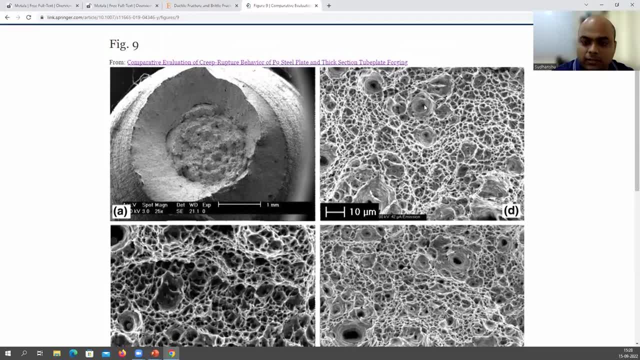 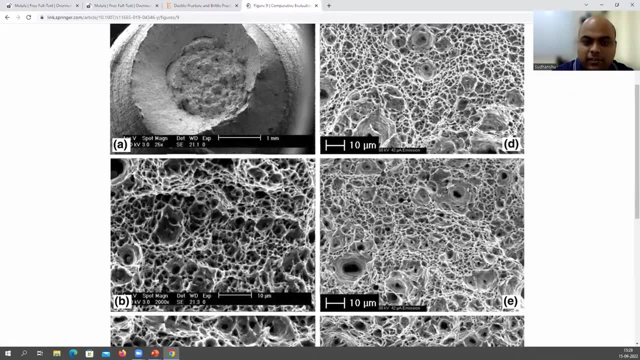 dimples, then you have very close dimples here. okay, and if you see, you can see some inclusions of second phase particles, isn't it okay? so this is how you can see the difference between the two. okay, so this is how you can see the difference between the two. okay, so this is how you can see the difference between the two. 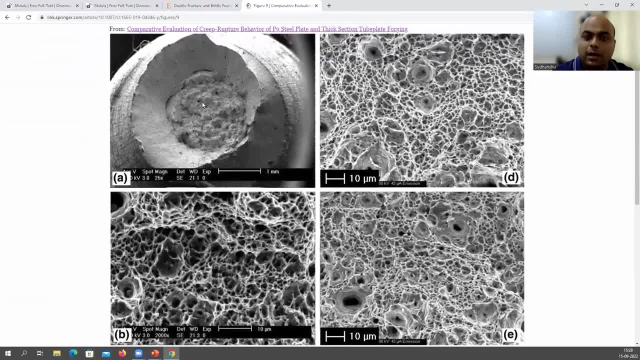 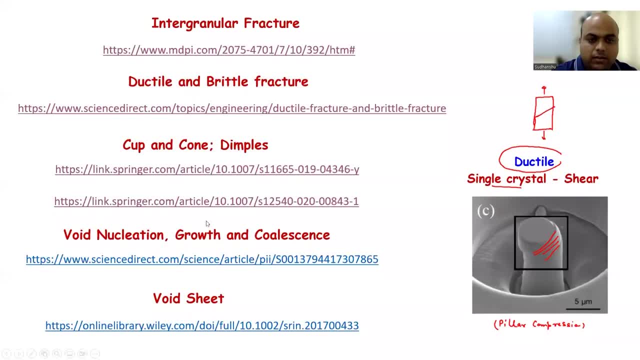 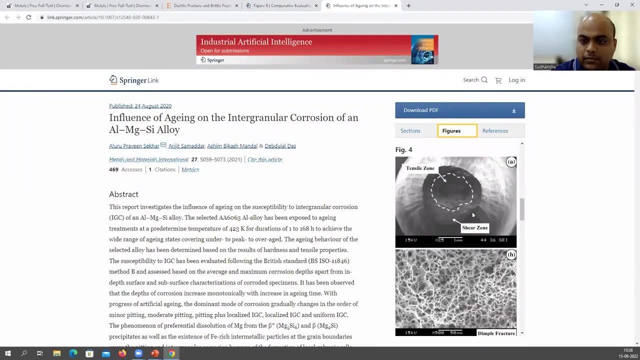 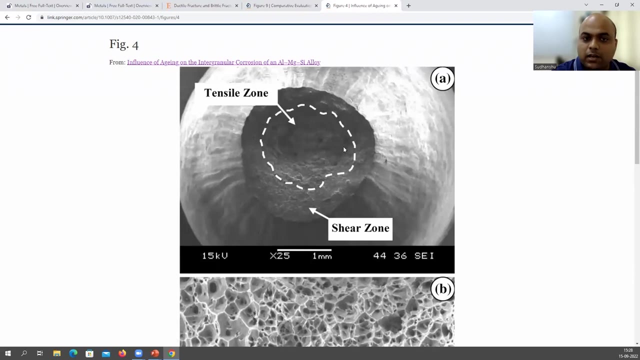 your dimples are going to look like, and this is typically cup of cup and bone fracture. so there are two parts: cup and cone. so this is like a cup. okay. now the next is again cup and cone. so here is this one, okay. so again you see a cup here. so you have fibrous zone at the center, this part here, and 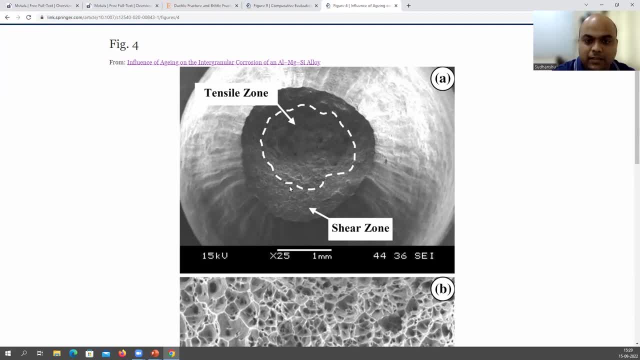 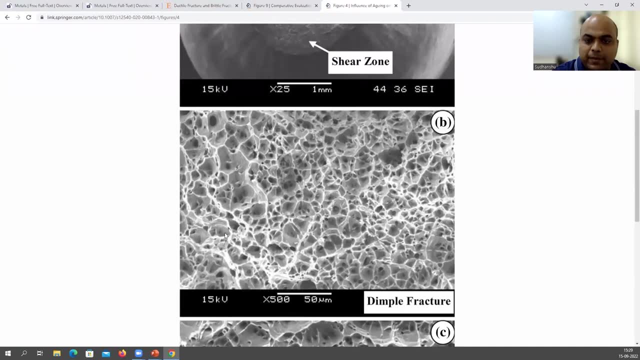 and then you have shear zone or shear lip in cup and cone fracture And if you see, if you just magnify this particular region at the center, the fibrous zone, you are going to observe dimples like this. okay, And you can see the inclusions right. 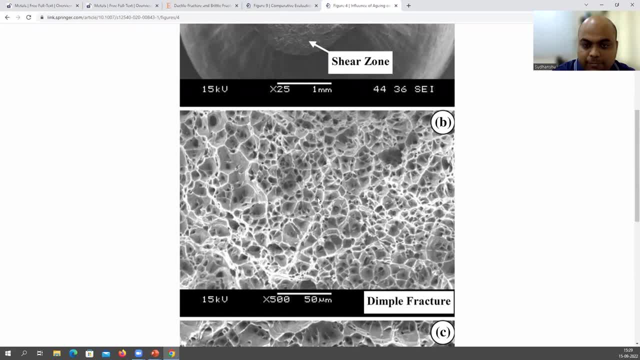 All these are inclusions. This guy here, this guy here, this small, small, you know particles, what you see, those are second phase particles or inclusions. We have discussed that Voids are going to nucleate at these locations. 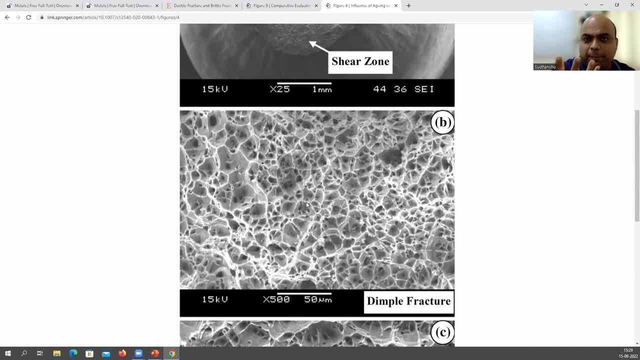 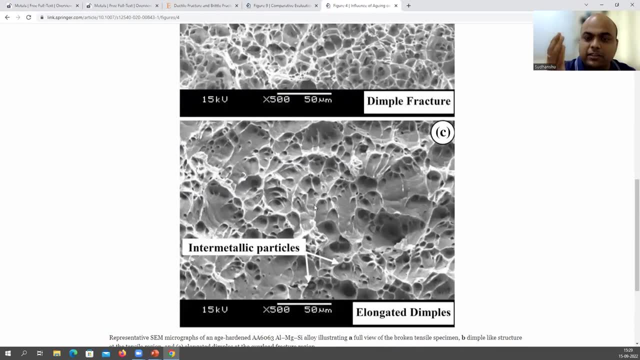 So this is at the fibrous zone where you typically see EQS dimples. We discussed about this. right Now, this is in the shear lip, where you see not the EQL. it is like elongated. You can see it is elongated dimples, okay. 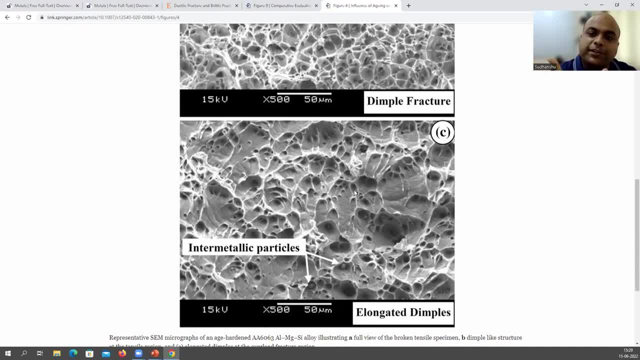 So if you are in the fibrous zone, typically you are going to see EQS dimples. If you are in the shear lip zone, then you are going to see elongated dimples. as I have shown, You can see also the intermetallic particles here. 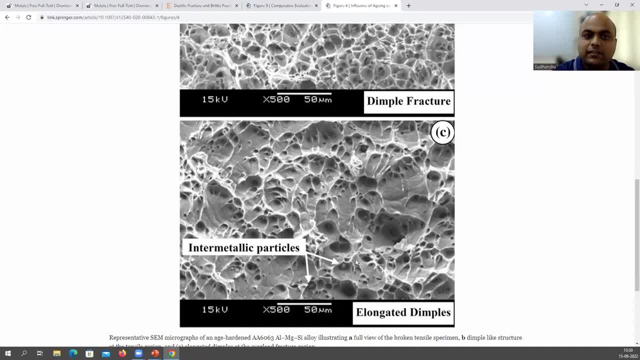 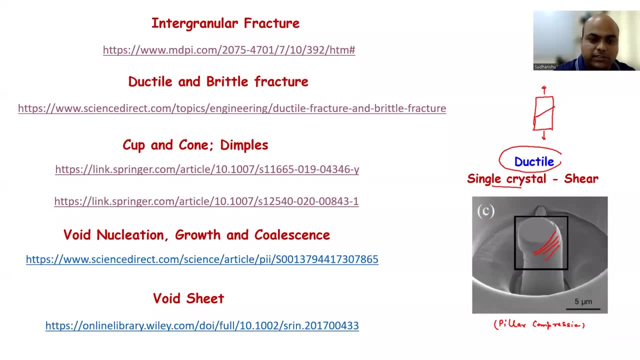 One is this side, another one is this, another one is this. okay, So I have shown you top and cone failure, as well as dimples and inclusions. Now let's see the schematic of void nucleation, growth and coalescence. 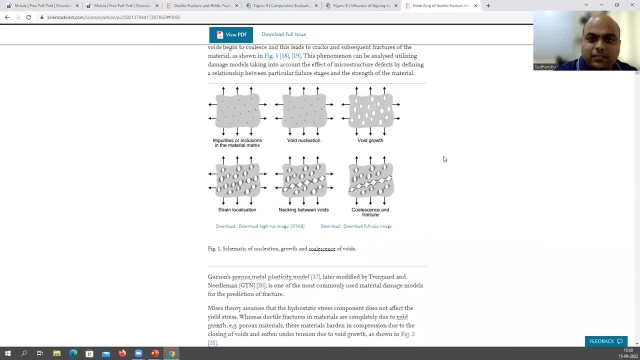 Okay, So this is a nice schematic. okay, You can see the impurities or inclusions Voids are going to nucleate, then they are going to grow in this stage. okay, Then what you have? what happens here? you have a strain nucleation between these two voids. 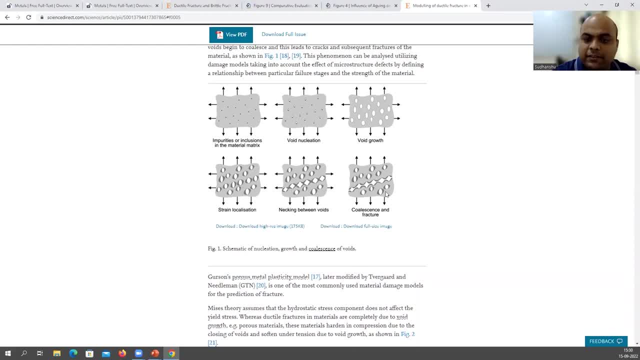 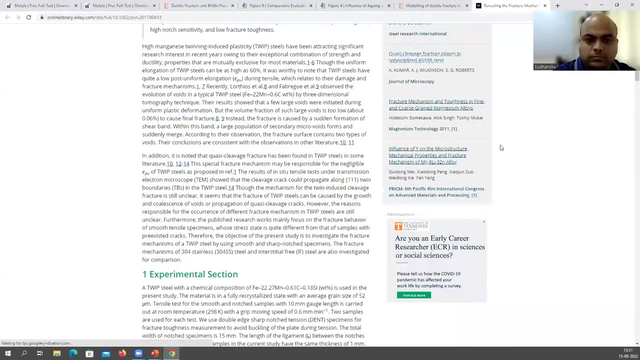 So because of the strain nucleation it grows and then finally it coalesces, right? So this is also we discussed. I just wanted to show you a schematic for better understanding Now. the next is void sheet. So here you can see very nicely void sheet, right. 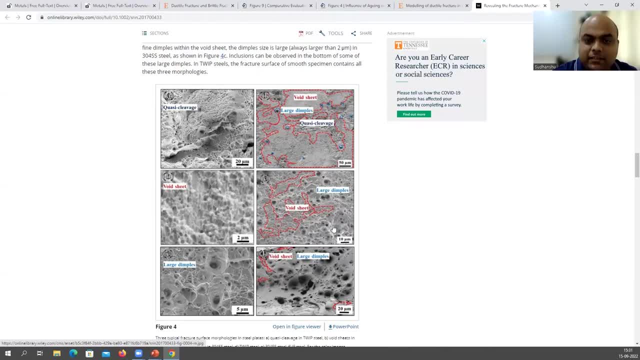 So you can see large, large dimples. see image E. you can see large, large dimples all around, but you also have very small dimples in the red regions here right Inside the red region. So these are void sheets and then you have large dimples. okay, 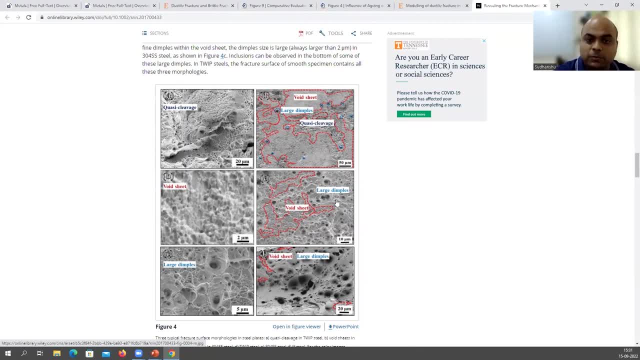 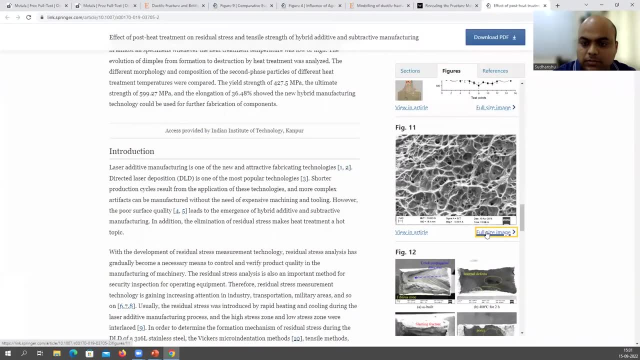 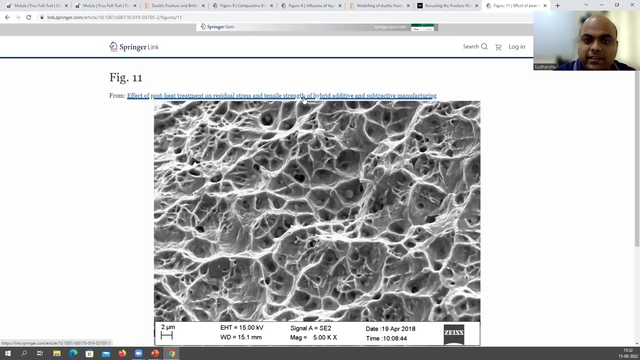 So this is like void sheet mechanisms We discussed. We talked about this before. Now let's see dimples and inclusions. This is a very nice image actually, This one. So this is from a paper titled Effect of Post-Heat Treatment on Residual Stress and 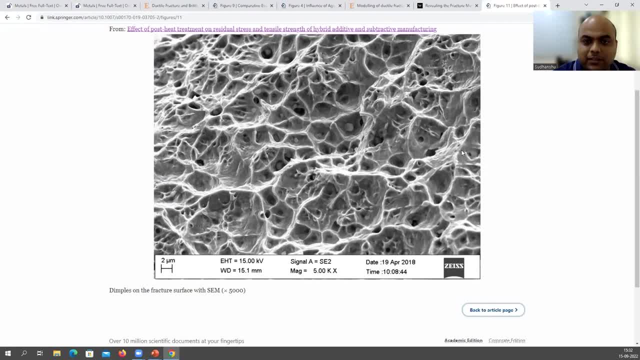 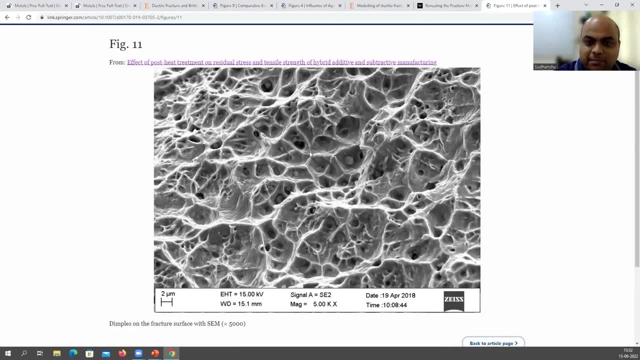 Tensile Strength of Hybrid, Additive and Substructive Manufacturing. You can see very nicely dimples and then lots of particles, isn't it See? all these are second phase particles And each dimple should contain one particle. 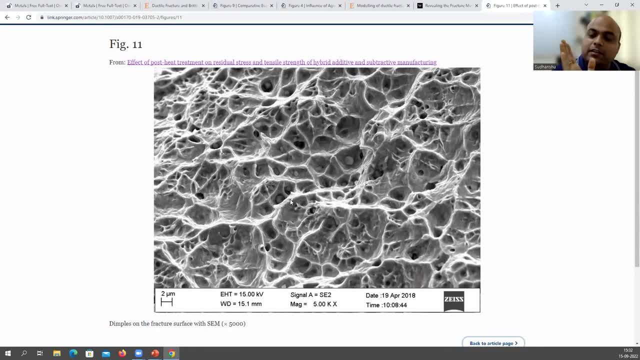 That is what we discussed. So wherever you are not seeing here, you will see on the other side of the sample, fractured sample. okay, So see, this is one inclusion, another one, another one. So everywhere you can see the presence of second phase particles or inclusions. 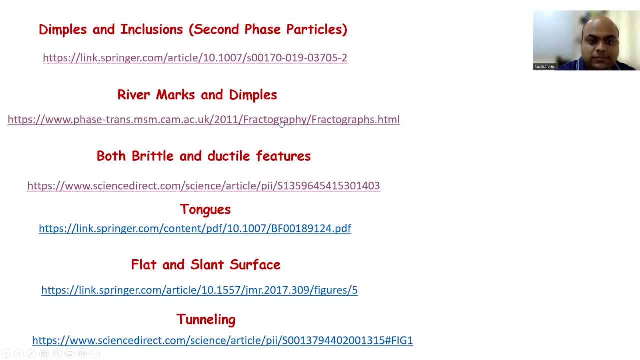 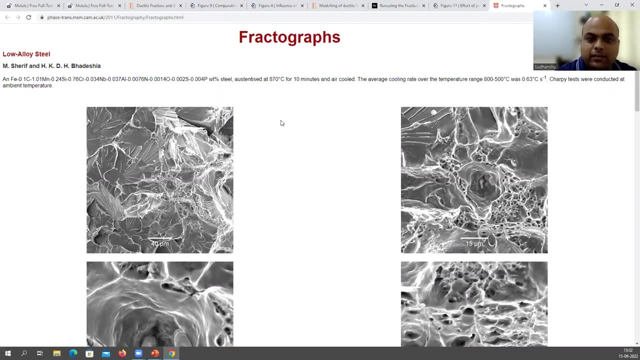 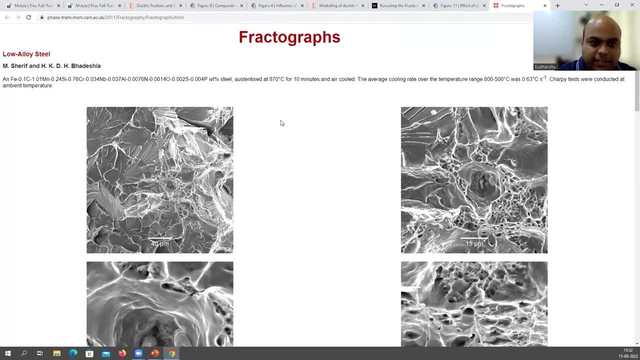 some of the phatographs for steels. Okay, So what you see here on the left side, these are river marks. Okay, all these lines, all these lines, These are your river marks. Okay, Very nice image. You can see lots of river marks. 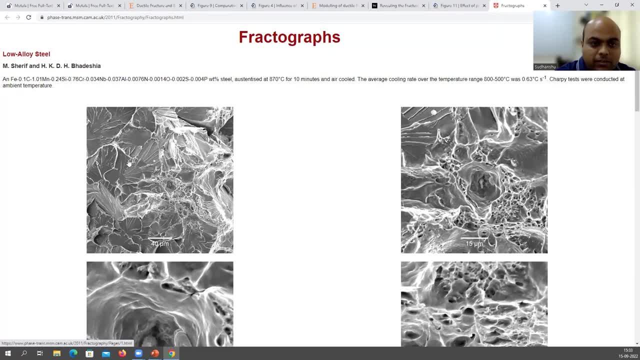 And these are your facets, facets, Okay. all these are one facet. This is one facet Again. this here is one facet, Okay, And each facet are going to contain river mass. that is what we discussed. this one on the right side shows you. 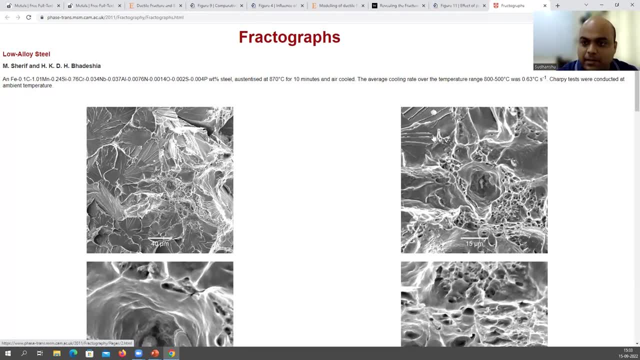 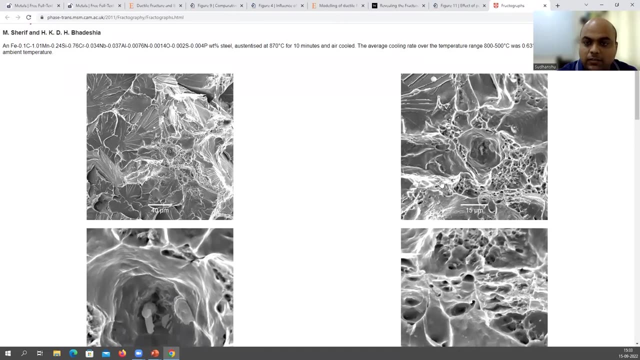 mixed fracture where you can see cleavage, river mass pattern here, right. but you also see dimples, see in this region, okay, and inclusions also here. if you see this is a very large dimple which contain inclusion shown here, okay. so you have dimples, you have river mass or say cleavage. 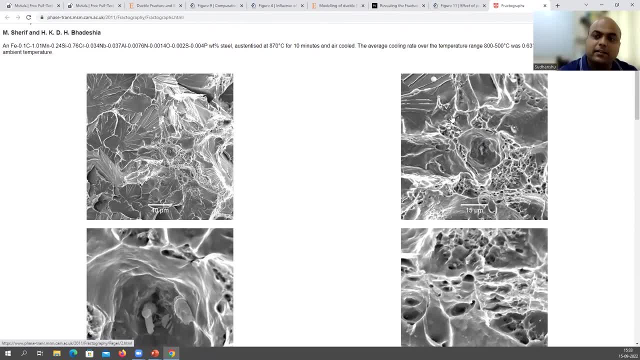 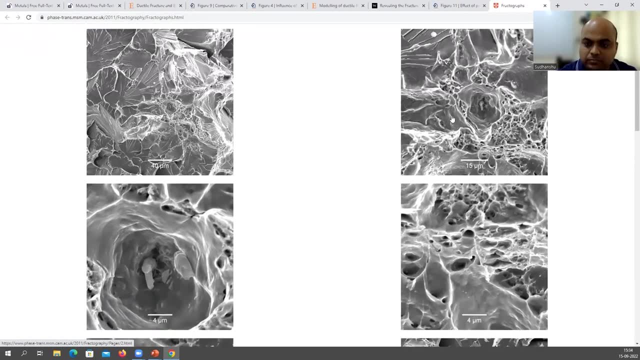 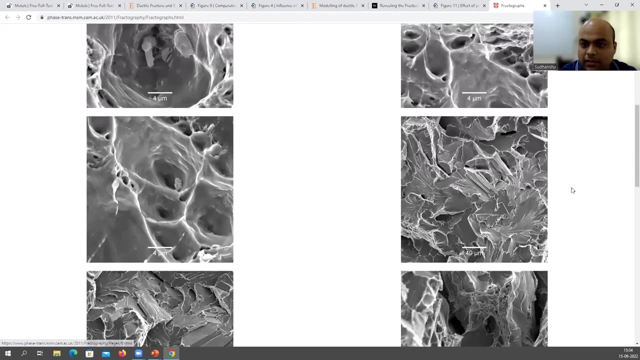 pattern. so it is a mist type failure. it is nine. it is a mist type. that means it contains both ductile feature as well as cleavage feature. okay, all these are dimples. these image here also. this is dimple now here. what is this? so this is your cleavage fracture. right, you can see. 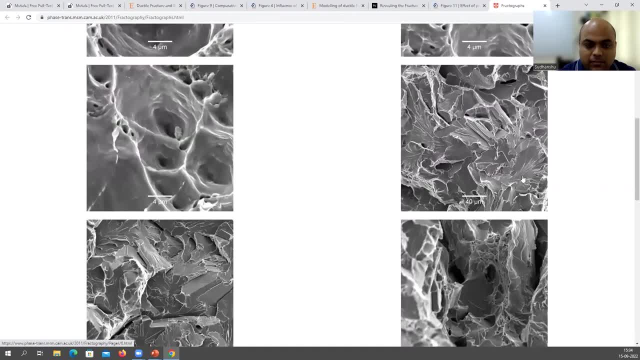 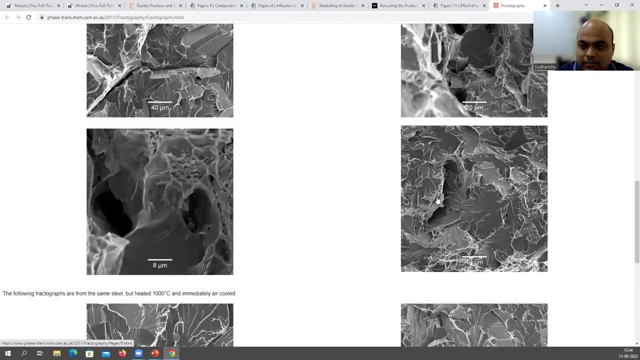 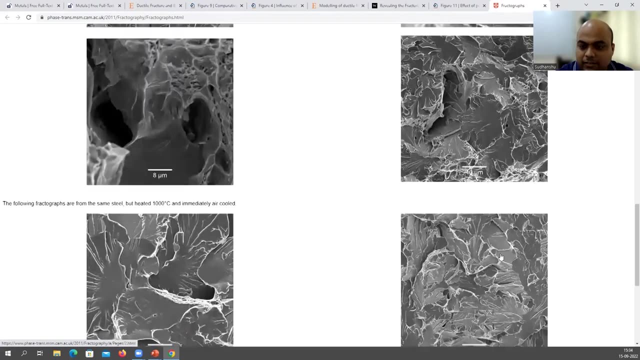 river markings. all these are your even marks. okay, again, this is also cleavage fracture, not here? also river marks, same river marks. you can see lots of river marks. so this is one facet here. i would say another facet here. okay, so all these are examples of river marking and cleavage fracture. 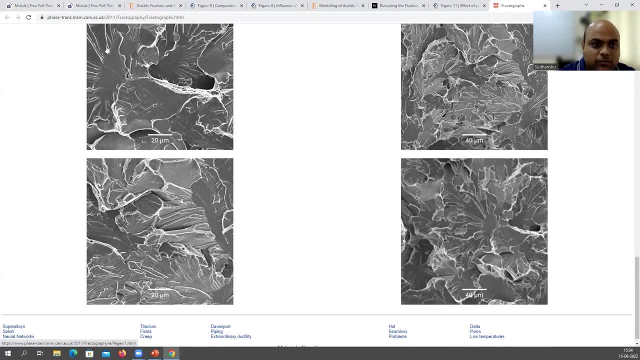 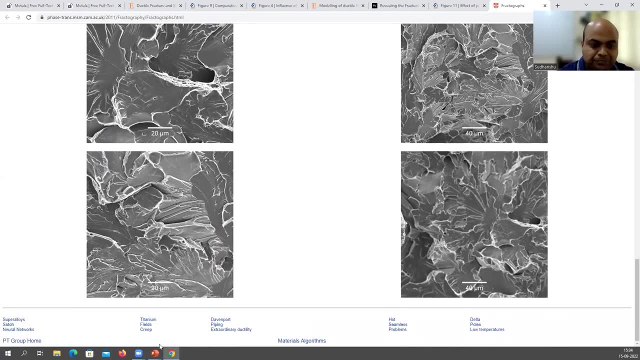 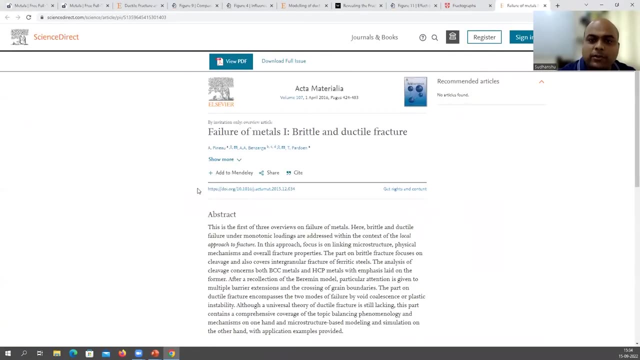 okay, so you can see one facet here. this is so very nice image of river martin. again, all these are mars, river, mars, okay. okay, now let's see both ductile and brittle features. so in this paper you are going to see lots of images. so this is from alta materialia. 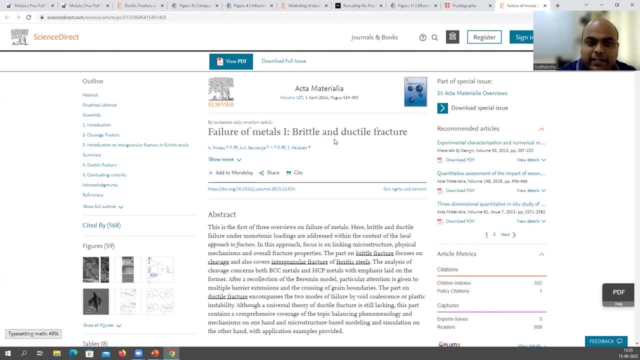 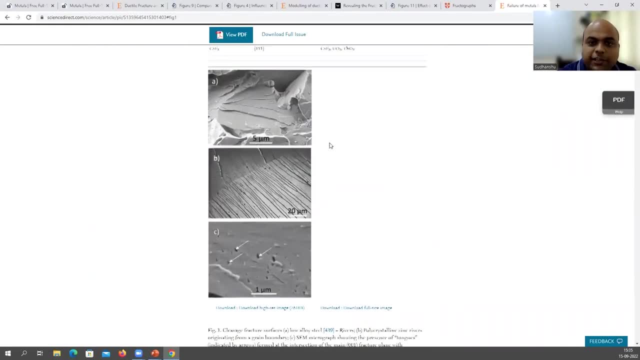 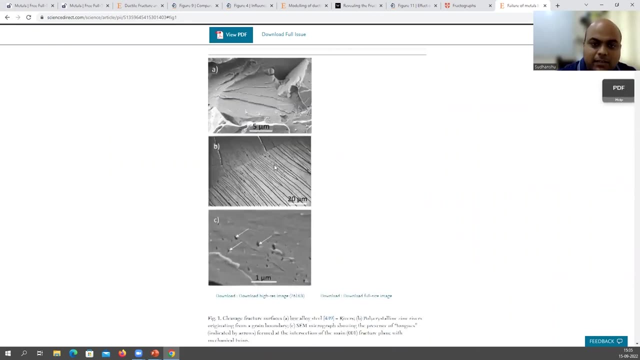 fatigue of metals: one brittle and ductile uh fracture. so this is an overview article, okay, so what you see here in image a, these are your river marks and this is the facet right. so it's a cleavage fracture. this is again another river mark. okay, so this is for. if you see at the bottom, this is for low alloy steel. 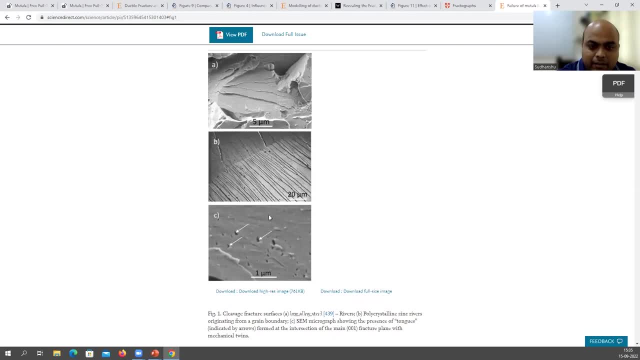 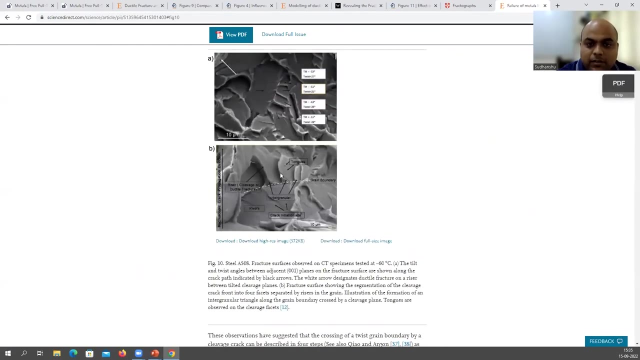 and this one is for polycrystalline zinc, number b and in c. you see tons, okay, we also discussed about tons, so these are tons, okay, okay, so this is the uh low magnified image. you can see tons here. very small features, right, okay? 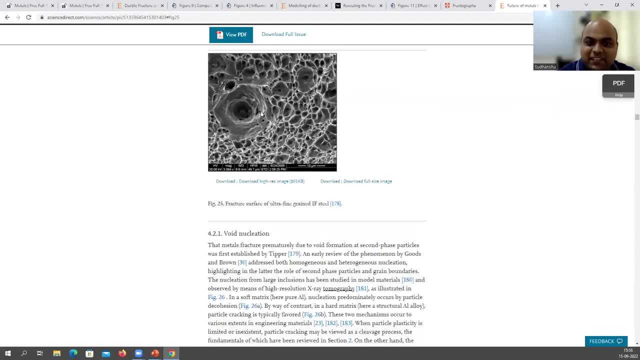 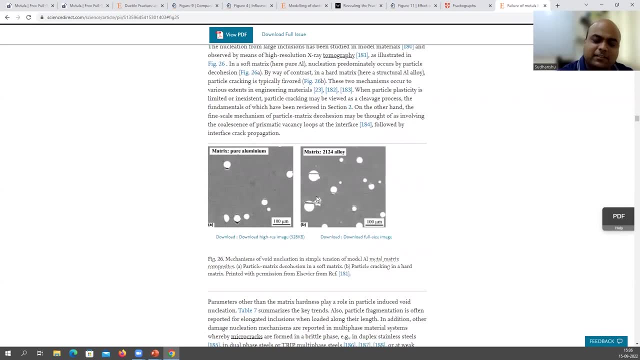 so, uh, what is this? gimpels right? so ductile failure. okay, so these two images, these are actually for composites, metal matrix composite, but if you assume it to be, you know, second phase particles in a given alloy, it nicely shows the deep bonding as well as fracture of the particle. so assume that these are. 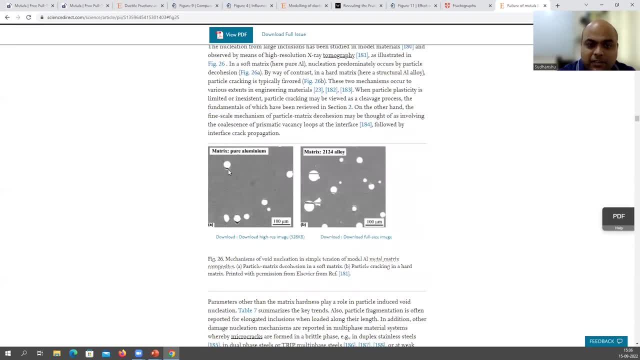 are particles, white particles. So you can see, in the first one you have debonding at the interface and in the second one you have the particle fracture. and this is what we discussed. It depends upon the nature of the interface, right, It can either debond or you can see the fracture. 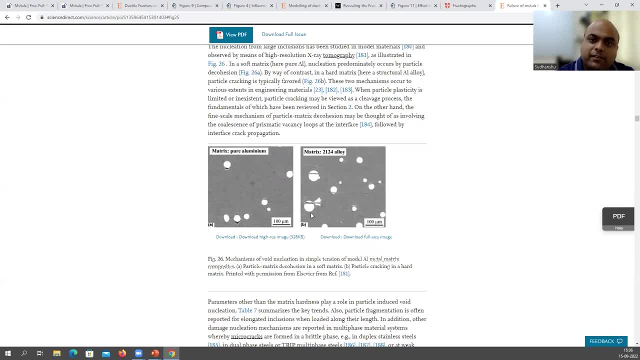 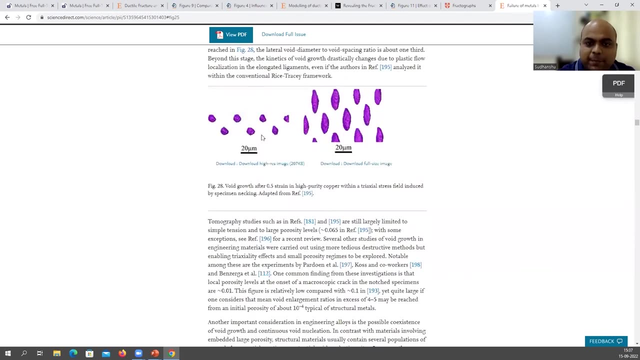 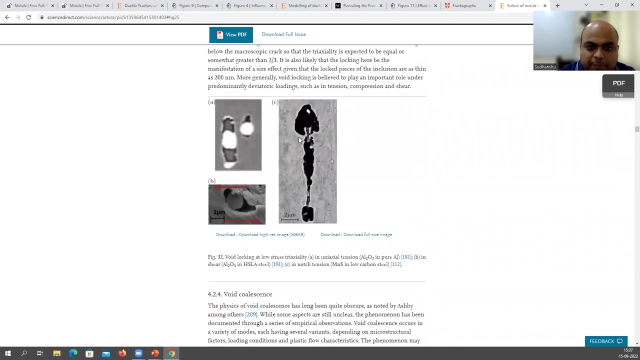 of the particle themselves and from there the voids are going to nucleate. right, This is how voids nucleate in a given ductile alloy or metal commercial. So these are typical images showing, you know, void nucleation and then void growth. I wanted to show you another image, Yes, so here. 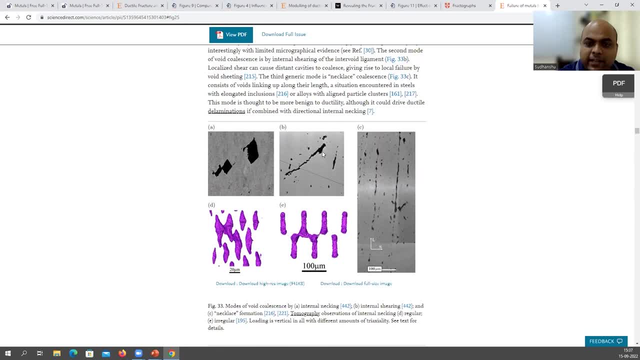 So you have these voids, they are going to grow and then they coalesce. You can see very nice coalescence here. okay, Similar here. You can see void coalescence in this particular region. Similarly, voids are going to coalesce. 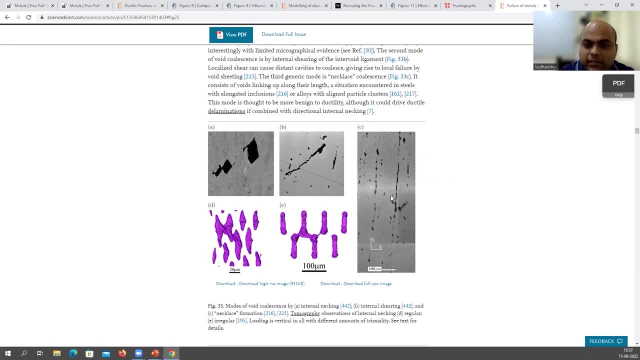 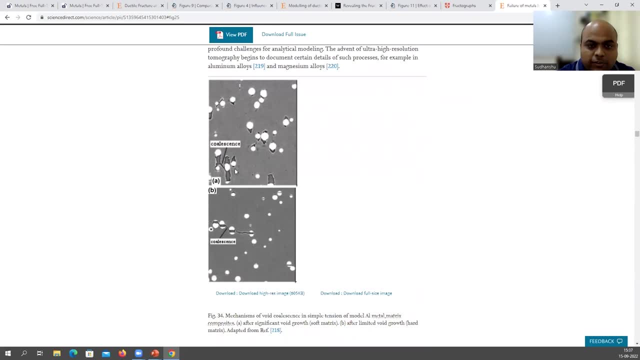 in this particular region. See the arrow here. okay, Here also voids are going to coalesce right. Here also you can see voids were formed mostly in image A, mostly because of the debonding right. And then you can see at the bottom, left bottom, and see the arrow you can see. 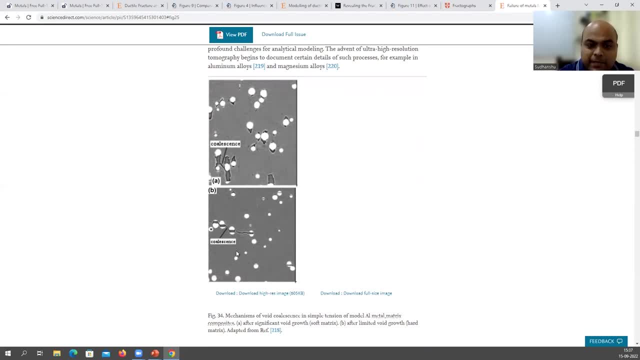 coalescence of those voids. Right in image B the voids are nucleating, mostly because of the fracture of the particle, and then they are also going to coalesce right. So this is how voids nucleate: they grow and then coalesce. 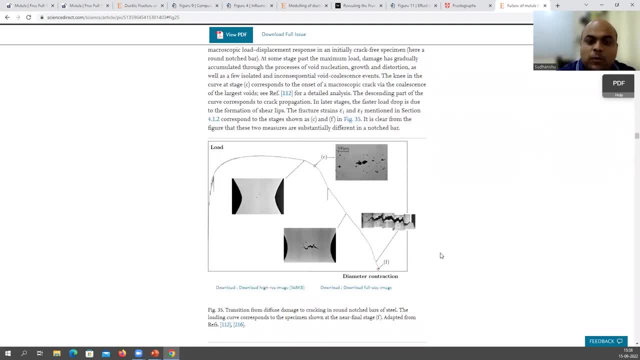 Okay, this is also a very nice image which shows how your voids are nucleating and growing in uniaxial tension. Remember when we were discussing about top and cone fracture, I mentioned that after necking or during necking you see lots of voids right And you can see here. So 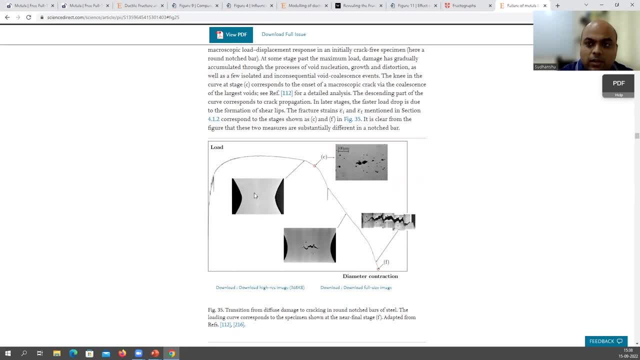 all these, the dots here in the image see the arrow. these are voids, okay, And as you increase the load or not increase the load, as you increase the strain, you are seeing that the voids are going to grow. That is image C here. okay, And after some time they are going to coalesce, right, And 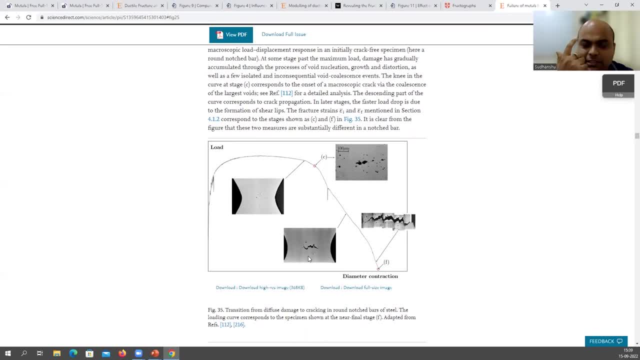 they are going to form cavity or the crack inside. Just remember what we discussed during top and cone fracture mechanism. okay, Now this is also going to grow and finally you will end up getting a very thin sheet or ligament and that will lead to the shear lip, if you remember. 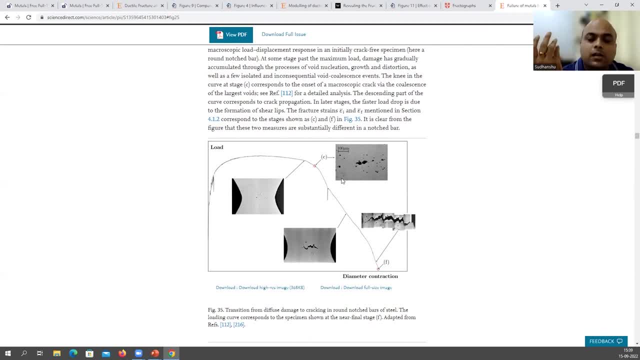 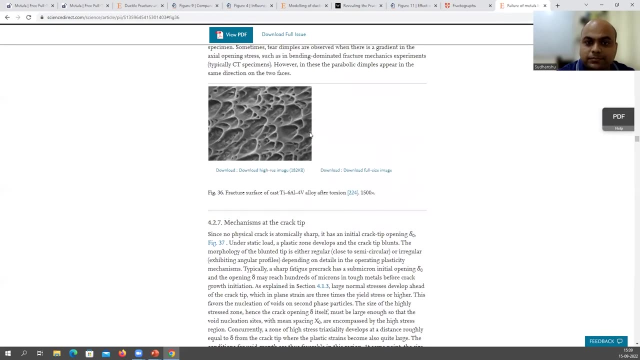 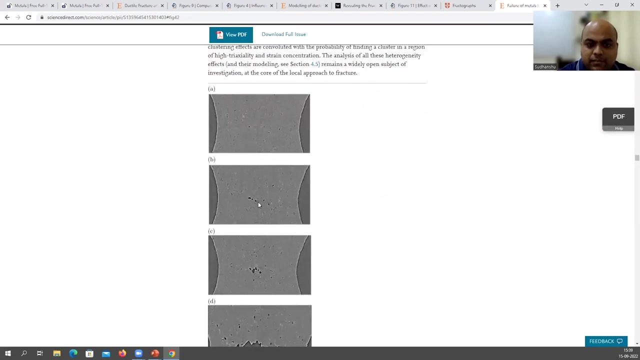 right. So this very nicely shows how you know voids are growing to nucleate, they grow and they lead to the formation of cavity during uniaxial tensile. So this is elongated dimple. okay, Same thing. so you have lots of voids in uniaxial tension. then these voids are going to grow You. 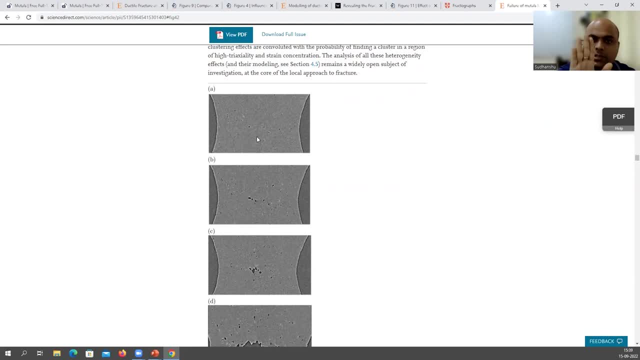 can see. this is at a particular location, same sample, and you are just doing tensile loading So you can see how voids are growing. the same voids. So you have this particular void. it is growing near voids. 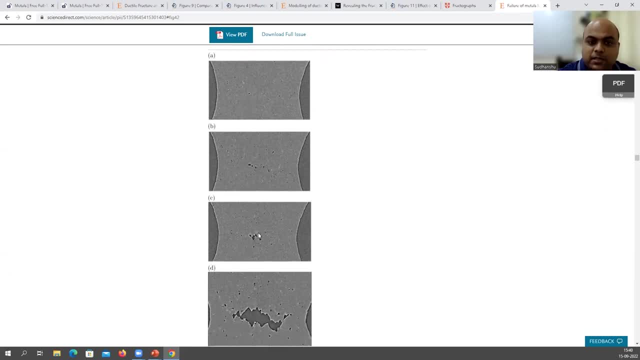 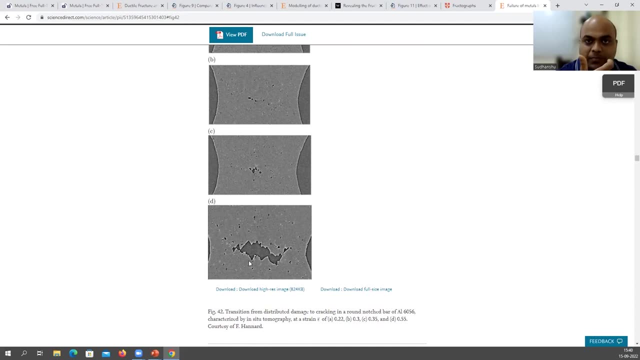 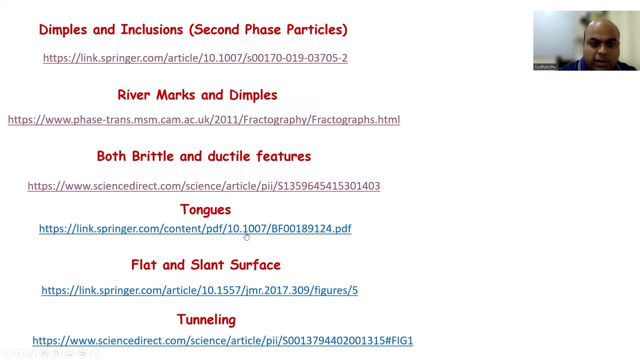 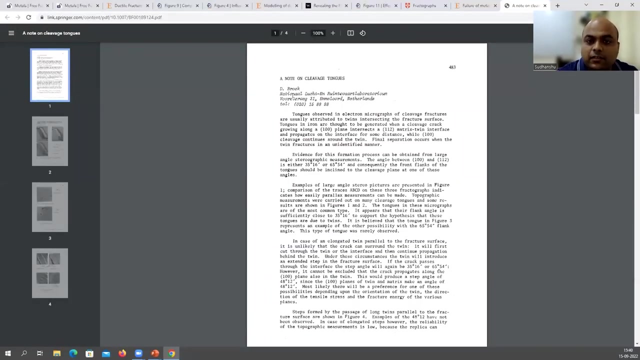 voids are also growing. now all these are getting merged coalescence and then then they also grow, leading to void, central crack right or cavity, and this is happening in uniaxial tension. okay, now i'll show you again tons. so it's a note of cleavage turns. okay, it was published way back in 1971, but it shows very. 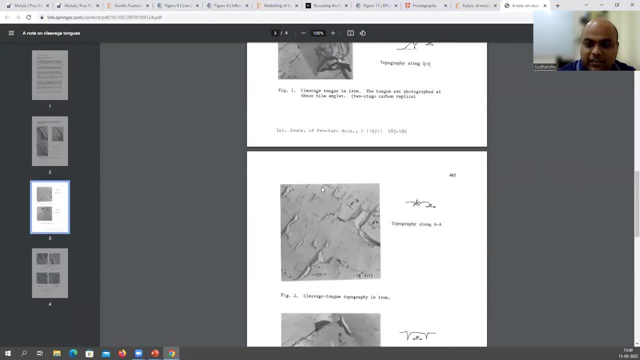 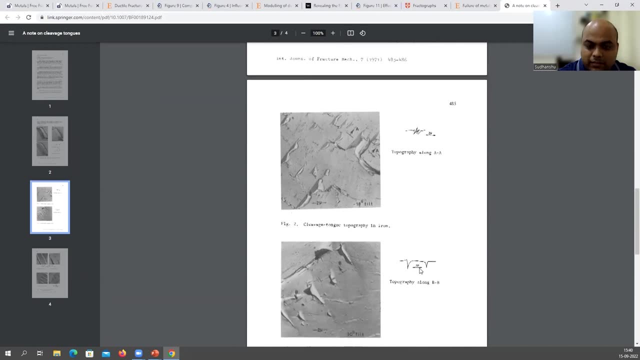 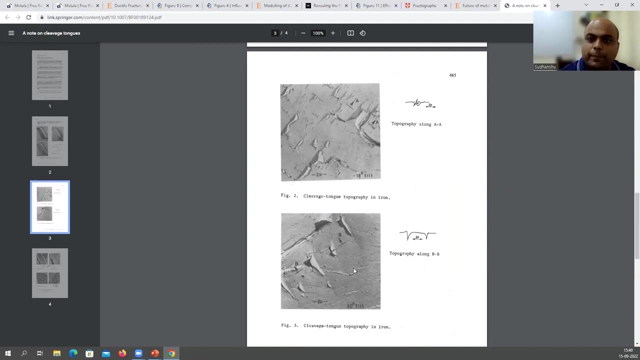 nice images of tons. so these are your terms in iron. okay, see, it's written: cleavage turn topography in iron. so these are your tons. okay, you can see all these are tons in iron. okay, and these are microstructural features, microscopic features, river martin turns- all these are microscopic features for cleavage traps. 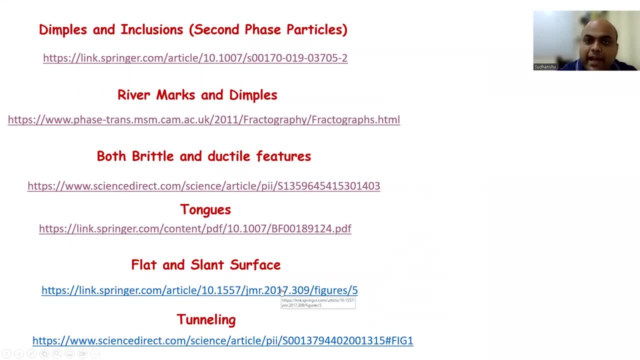 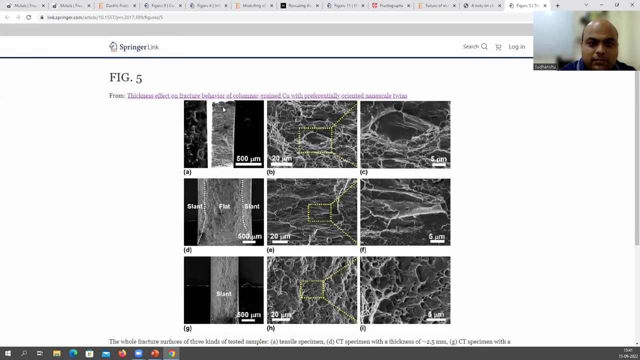 now, if you remember, we discussed about, uh, flat and slant surfaces tunneling, right, when we have a presence of crack during that type, track growth, right. so let's show, see those images. okay, so this is what uh, uh from the paper or the title is: thickness effect on. 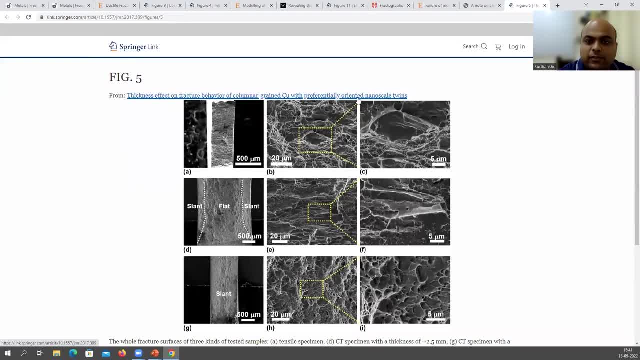 flat surface. so this is what, uh, from the paper or the title is: thickness effect on flat surface stretch of area of triangle drain proper with preferentially oriented nanostage points. okay, so this is for thicker sample. now we are talking about d image and g image bottom one. okay, so d. 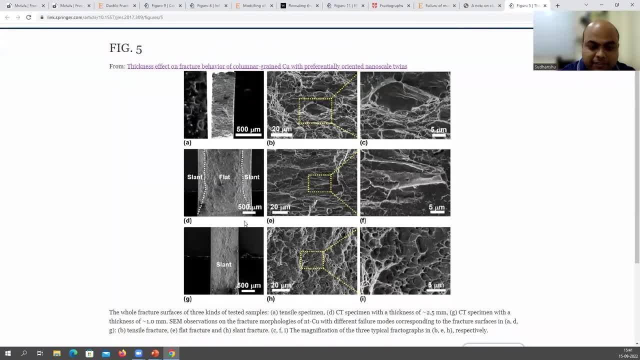 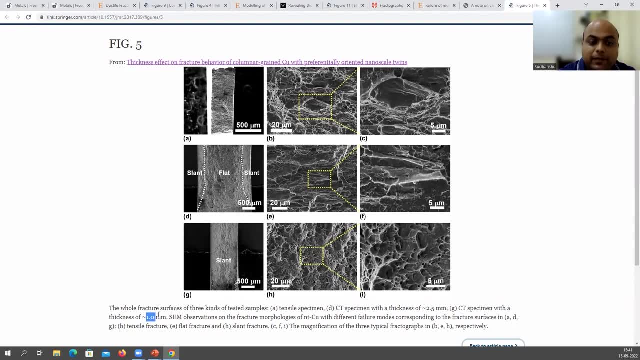 if you see it says land flat and slant, and if you see it is for 2.5 millimeter sample and the g1 is for 1 millimeter sample, right. so at 1 millimeter sample it is mostly slanting, as shown here. and if 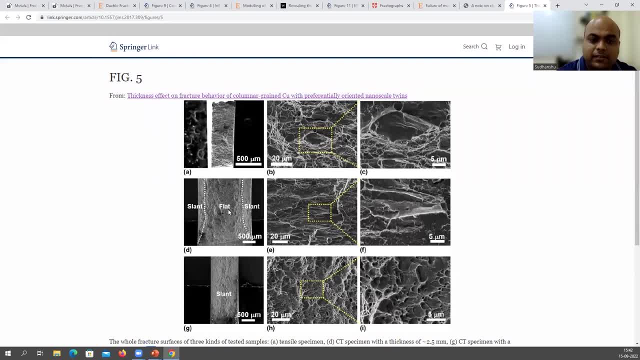 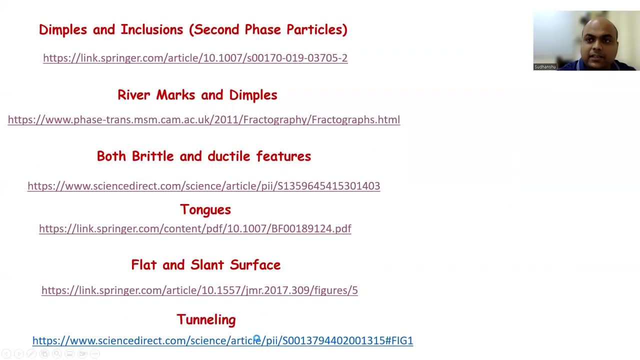 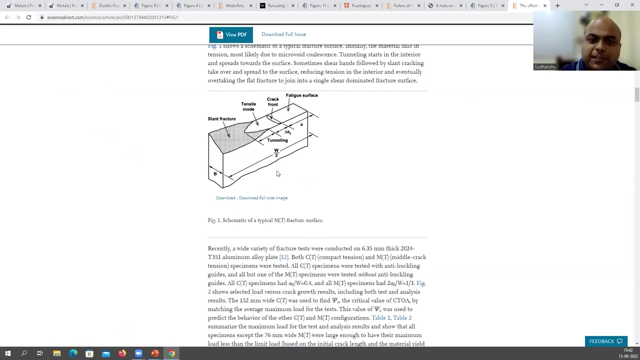 you are increasing the thickness, then you are also getting flat region. that is what we discussed, right, so you can nicely see slide as well as flat region here, depending upon the thickness now tunneling effect. okay, so this is the schematic. i also drew in 3d, if you remember. so this is your fatigue track. 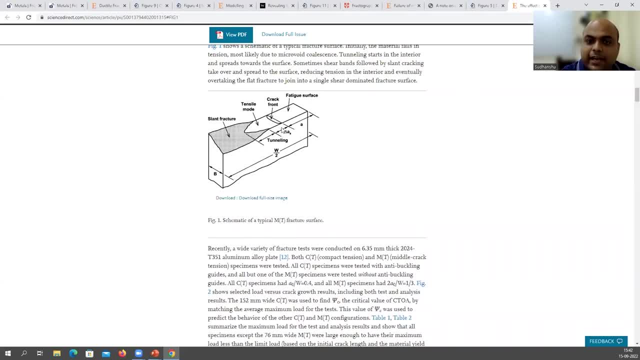 now track front profile. you can see it is like c type, okay, and it is growing. and it is growing higher at the center. okay, why? because of the tri-axiality effect. so void nucleation and growth becomes easier when you have tri-axial stresses, okay, or plane strain condition, which is existing. 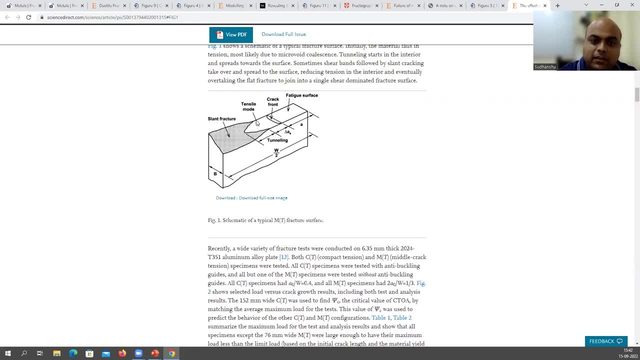 inside the sample or inside the specimen. okay, so the track profile. it looks like this, where the track length is higher at the center and it is the lowest at the surfaces. okay, and this is what tunneling effect is all about now. the last one is chevron patterns. 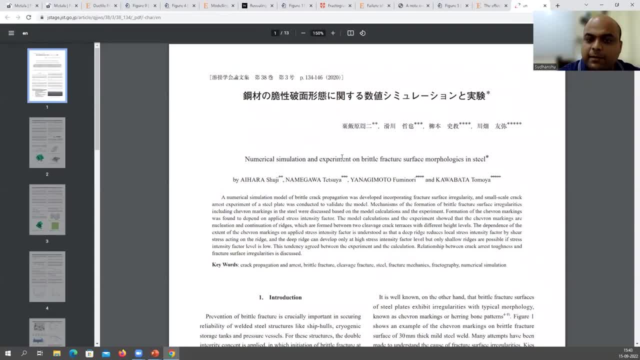 so this is from a paper called numerical simulation and experiment on brittle fracture surface morphologies in steel, and you can see very nicely the chevron pattern and it is the lowest at the surfaces. okay, and this is what tunneling effect is all about. now, the last one is chevron patterns.